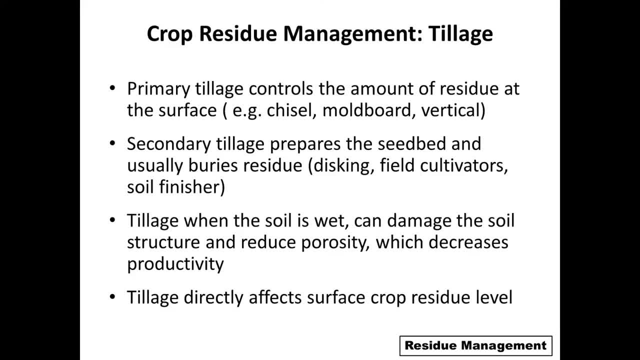 Any time you do any type of soil manipulation, you will be burying residue and affecting that soil in one way or another. There can be a lot of issues when we do the tillage. It's not just the type of tillage but also the timing of the operation, the speed of the operation, and so on and so forth. 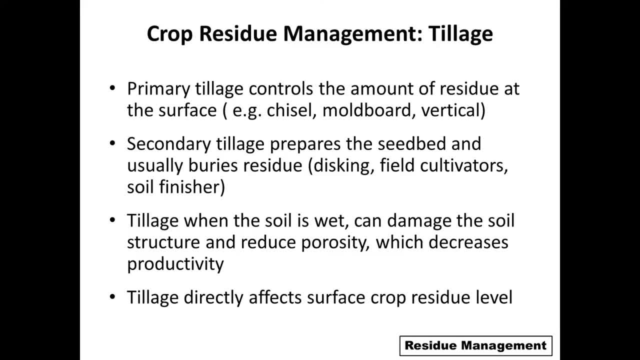 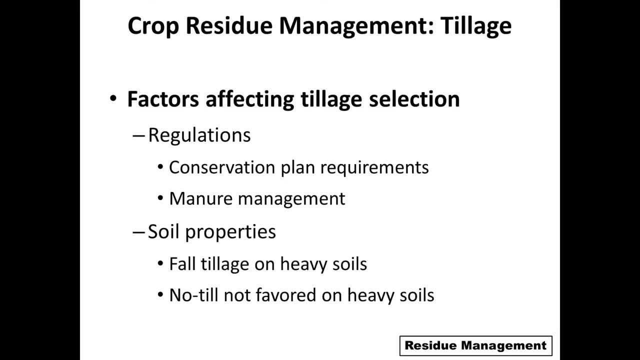 But the biggest issue is the time. The biggest issue is when we do tillage. when the soils are wet it can really damage soil structure and reduce porosity, which will decrease productivity, And also tillage affects the amount of residue on the soil surface directly. 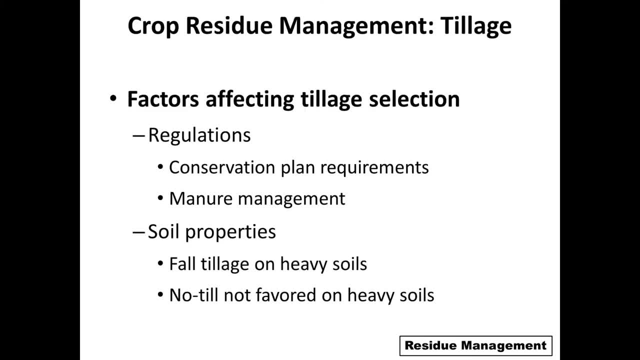 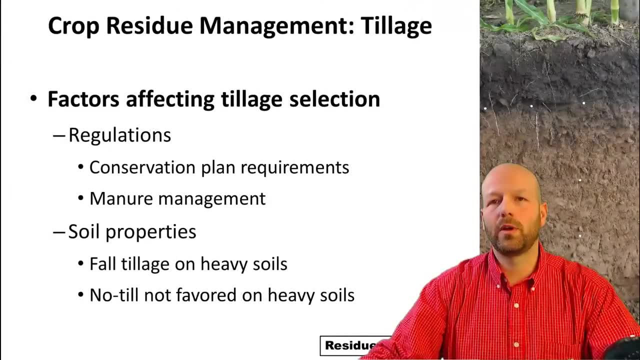 So one thing that is very important when we talk about tillage management is the type of tillage, or tillage selection, that we're going to do, And so there's a lot of factors that we must consider when we're looking at this. 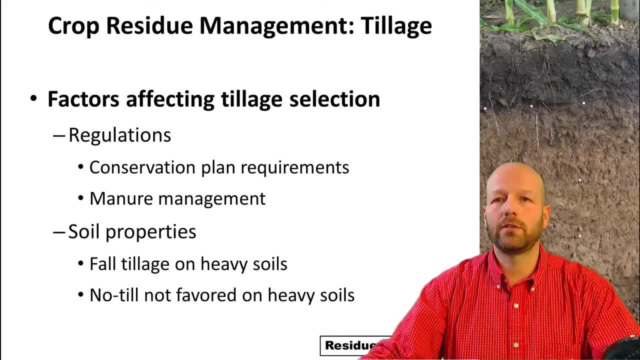 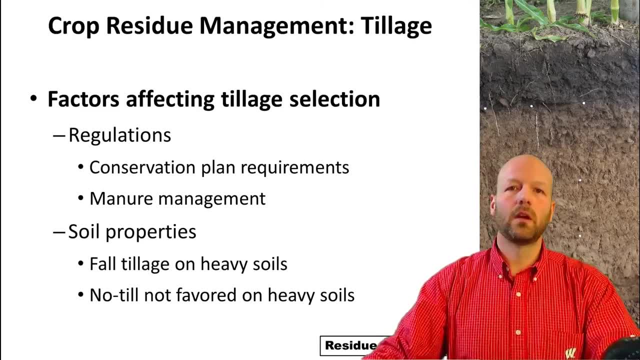 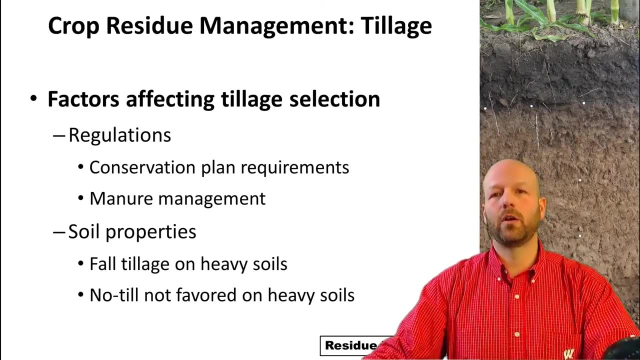 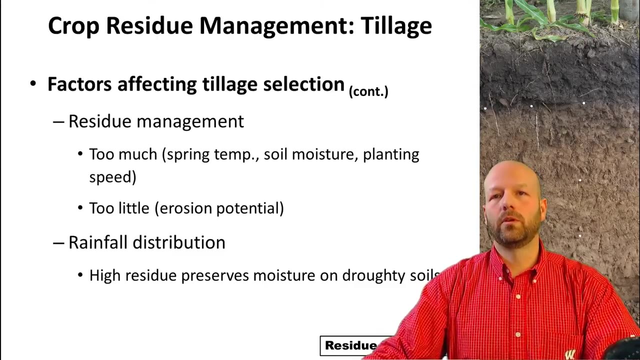 Obviously there will be some regulation requirements if you are having to follow a nutrient management plan, So there could be some conservation plan requirements too, But also your soil properties. What type of soil do you have? The slope of your soils and what have not will also have an impact on your selection of your tillage. 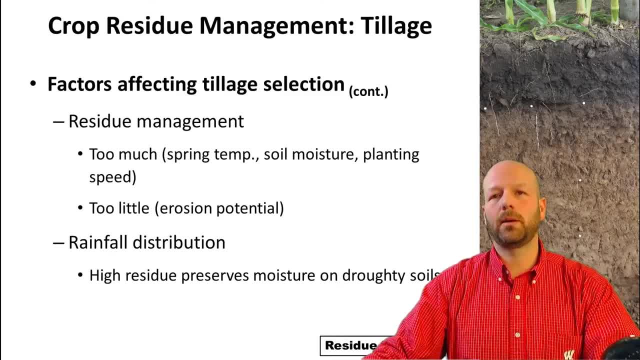 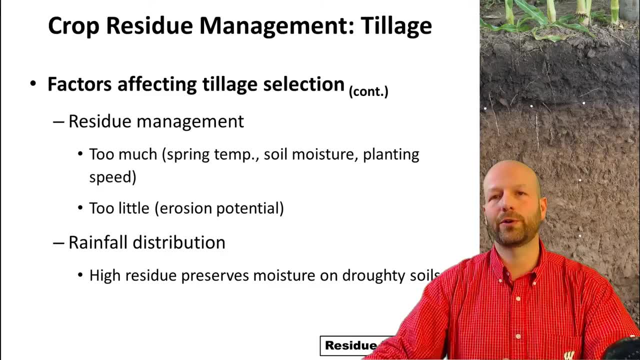 Residue management. it's usually seen as secondary, But it's also very important. But it's also a very important factor depending on your conditions and your crop management- scenarios such as corn and corn- That becomes crucial in those type of scenarios. 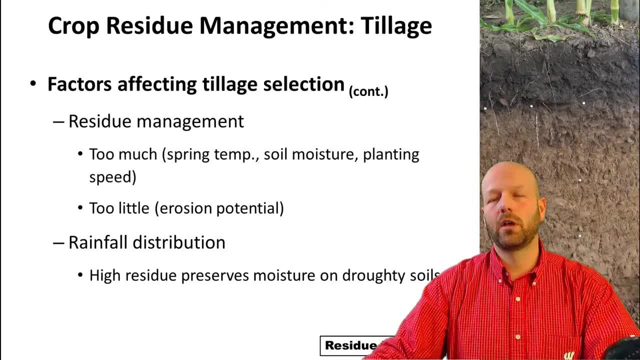 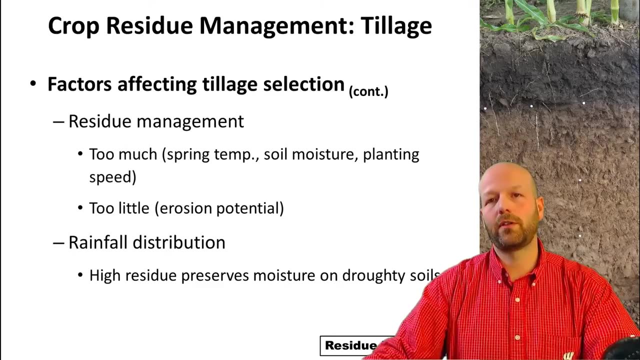 So things to watch out for would be the spring temperature, soil moisture- in the spring usually, but also during the growing season- And the interference with planting equipment. So the idea, or the logic behind it is that the more residue you have on the soil surface, 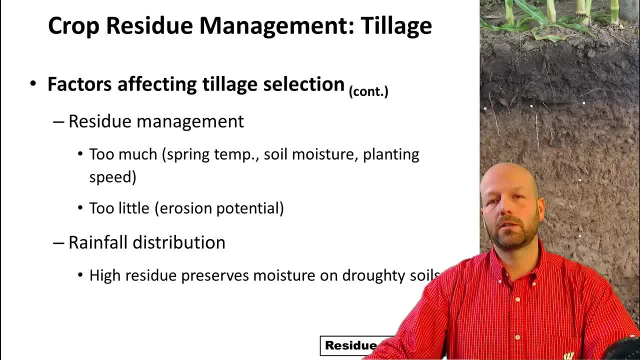 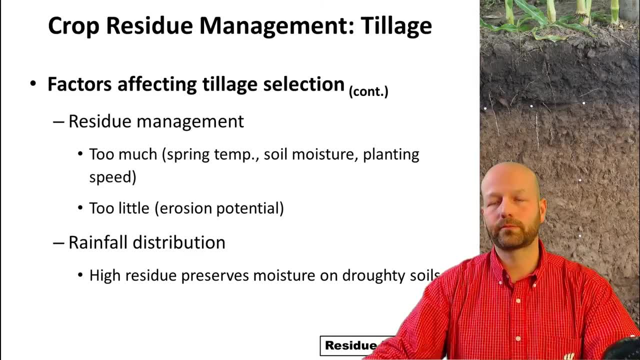 the lower your temperatures are going to be in the spring. So it takes longer for that soil to warm up, because less soil is exposed And so that residue acts as an insulation. However, when we look at the amount of residue, it affects also the amount of moisture in the soil. 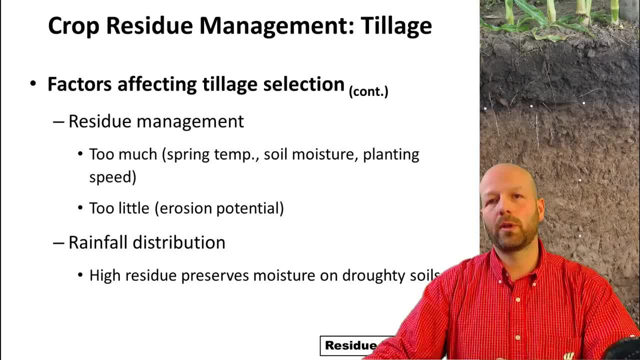 So the reason why soils in the spring warm up a lot slower, it's not only because of that they're exposed and the color and the effect of the sunlight hitting it, but also because that acts as a mulch. So if you have a lot of residue on the surface, it's not a good thing in the spring in a lot of conditions. 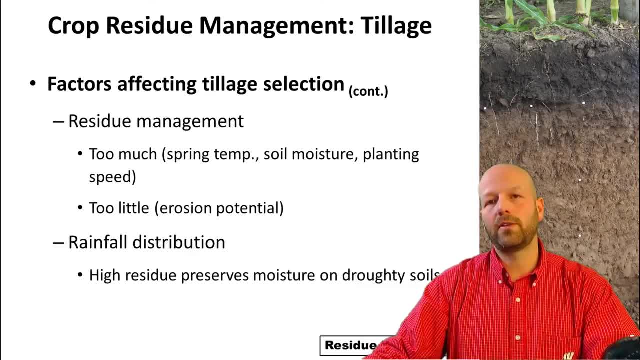 But then later on in the season when it gets hot and really warm, that residue again acts as a mulch and will keep a lot of that moisture in the soil And it helps water infiltration and a lot of other soil hydraulic properties. Too little residue in the soil surface also can lead to issues with erosion. 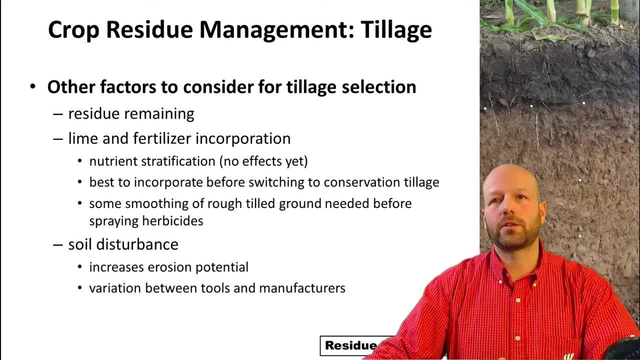 So there's other factors that can affect the consideration of what tillage to use, such as the amount of residue remaining. Again, this goes back to the crops you have in your rotation. Also, do you have the need to incorporate either lime or a different fertilizer or manures? 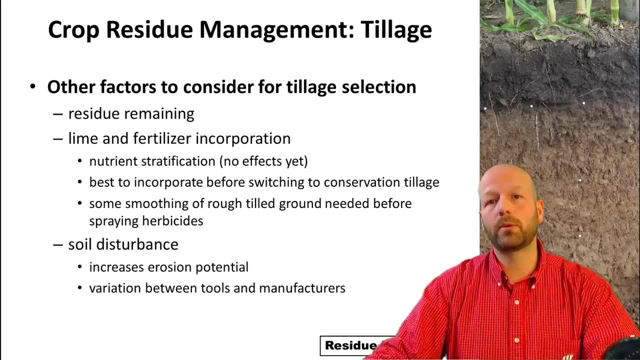 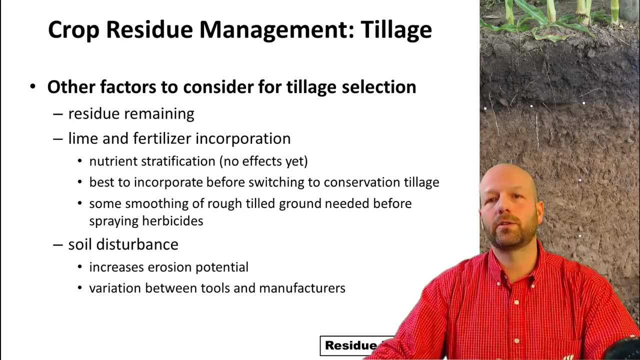 Some tillage equipment. it's better equipped or better at doing those type of jobs, But also have in mind that the soil disturbance increases erosion potential And there's a huge variation between manufacturers and the different tools. Not only that, also a lot of options that are offered can really change the way that a type of tillage equipment. 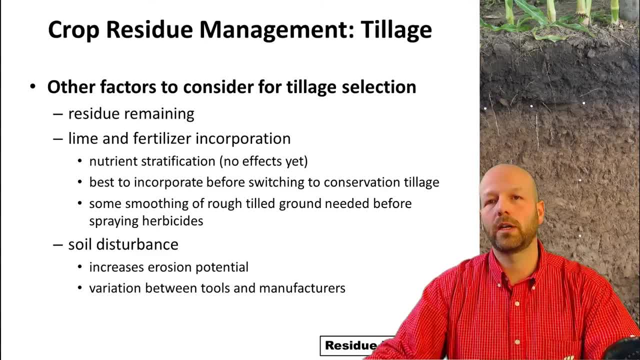 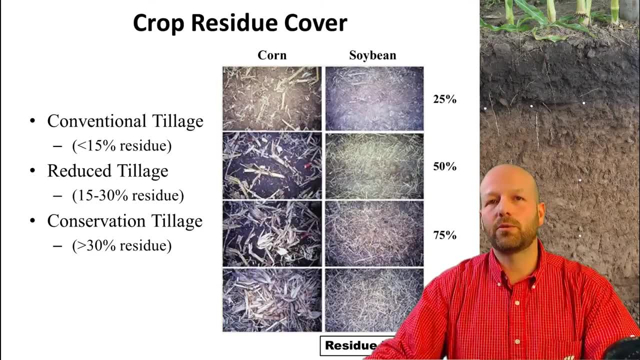 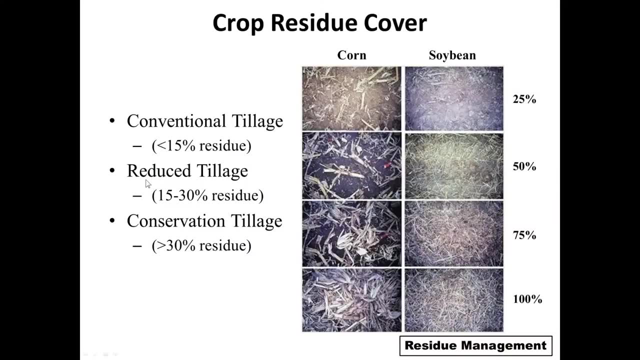 just specific tillage equipment can operate, can function in the field. Another way to classify tillage equipment is by looking at the amount of residue they leave on the soil surface. So usually we call tillage equipment reduced tillage, something that leaves about 15 to 30% residue on the surface. 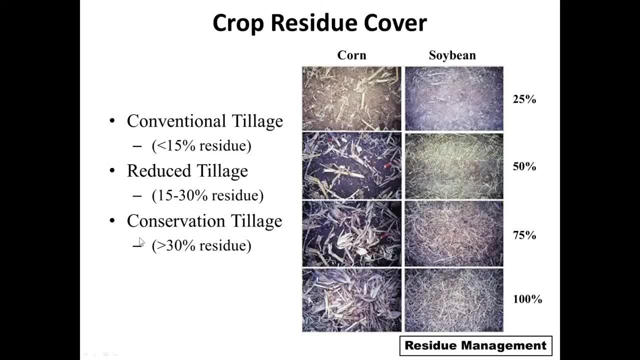 Something that leaves less than that we call conventional, And then something that leaves more than 30% residue. it's what we call conservation tillage, If you recall residue. 30% residue on the soil surface or more will lead to a decreasing erosion potential of up to 50%. 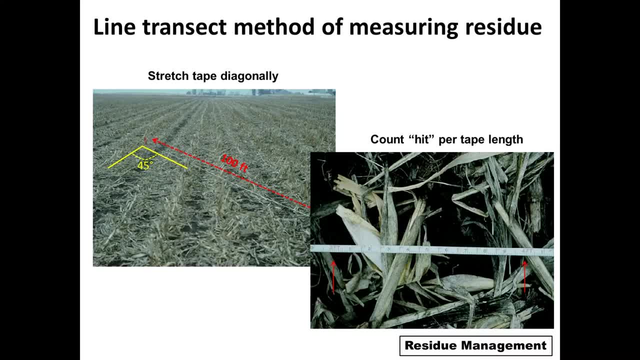 So that's why we call that conservation tillage. So how do we measure residues on the soil? We can use a method that's been used for a long time. It's called the transect method. So what you do with that is that you lay a tape measure diagonally across your rows in the field. 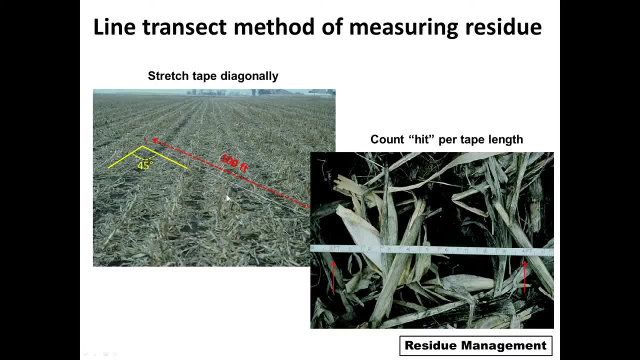 In this case, I have an example that we laid it out about 100 feet. You can do the same thing with a 10 feet section and do it several places in your field, And so what you're going to do is that you're going to count the amount of residue. 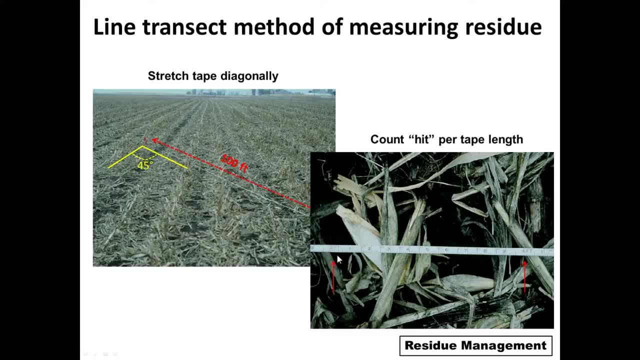 that hits that one foot interval. So in this case you see one foot. here at three feet mark, where I'm pointing, There's no really residue in there, so that would be a zero. Here at four we have some stalks and a little bit of leaves. 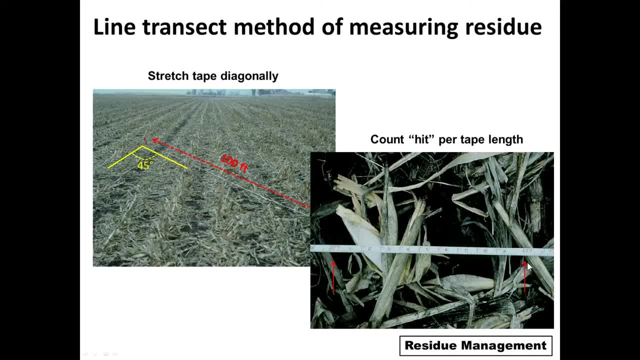 We call that a one, And so we add on that 100 foot transect how many hits we have, and then we add them up, And so if you're doing 100 feet, that would be your percentage. If you're using just a 10 foot section, you multiply that by 10, and that would give you the percentage. 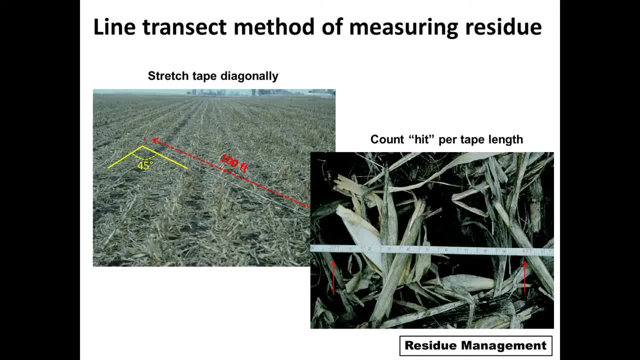 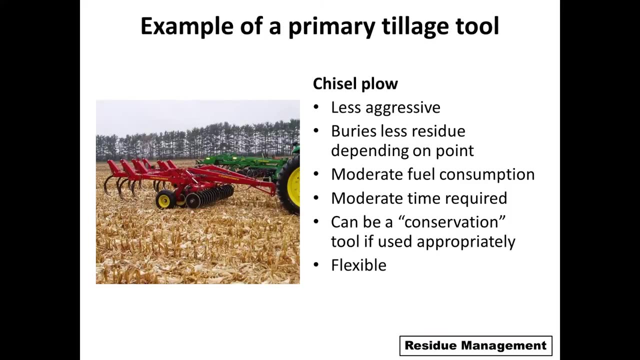 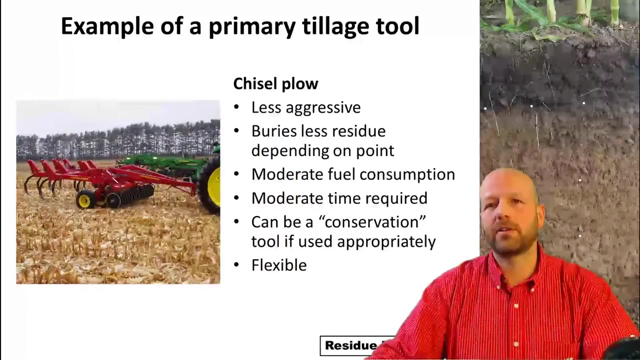 When we're looking at residue. you can count manure as residue. However, you should not count rocks as residue. So here's an example of a primary tillage tool very common here in Wisconsin: chisel plow. It could be less aggressive than other ones depending how it's set up. 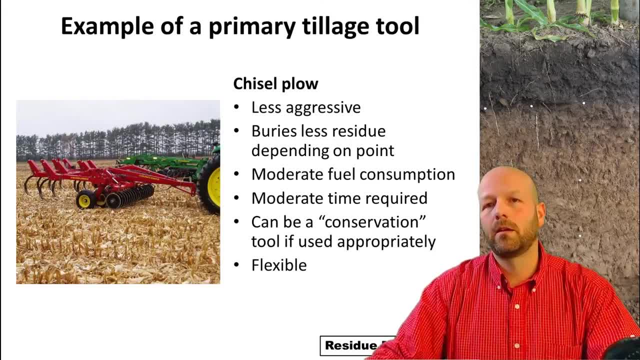 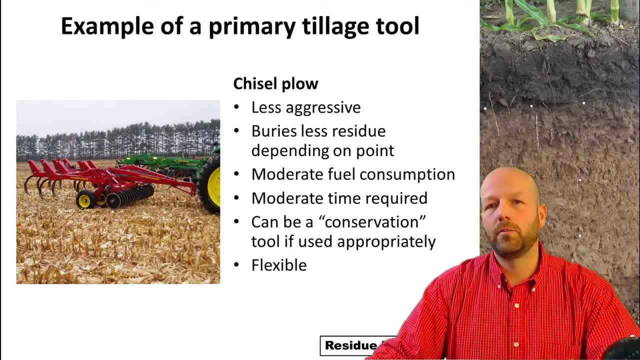 and this is a reason why I'm using this example just to kind of iterate this importance of the setup. It can bury less residue depending on the point or the setup of it Uses moderate fuel compared to other ones. It doesn't require a lot of time. 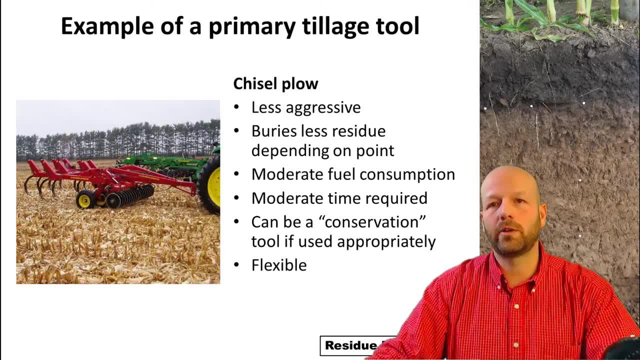 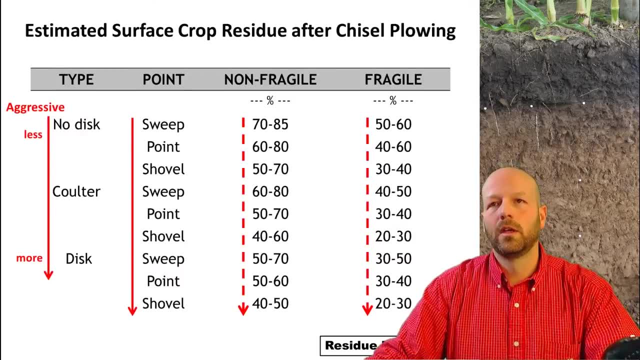 And if used properly or properly set up, it can be considered a conservation tool. So it's a very flexible tool and I think this is why it's so popular here in Wisconsin, so commonly used. So here's an example on the setup. 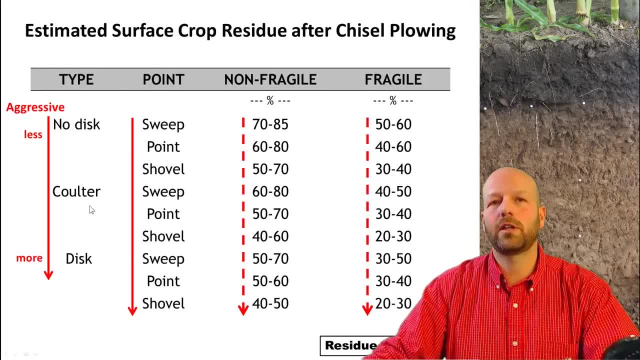 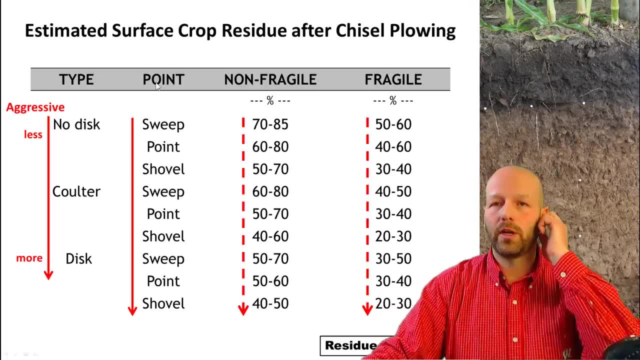 So what we're looking at here under the type section on the left is if it has discs or not. so no disc, a coulter and a disc, Then what type of point? going from sweep to point to shovel and then fragile soils and non-fragile soils? 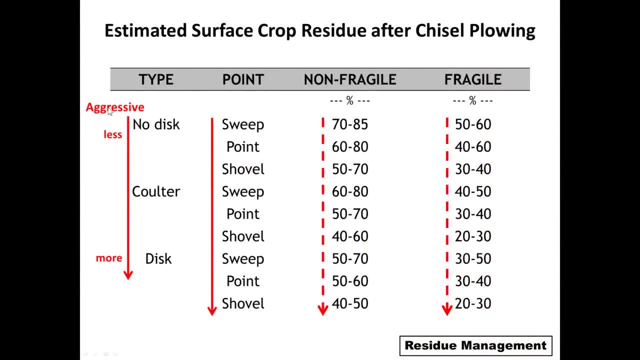 And the percentage here is the amount of residue left. and so I have included these red lines kind of showing off the aggressiveness of these setups, going from less on the top to more aggressive at the bottom. So you can see then, as you move from top to bottom, that less aggressive setup. 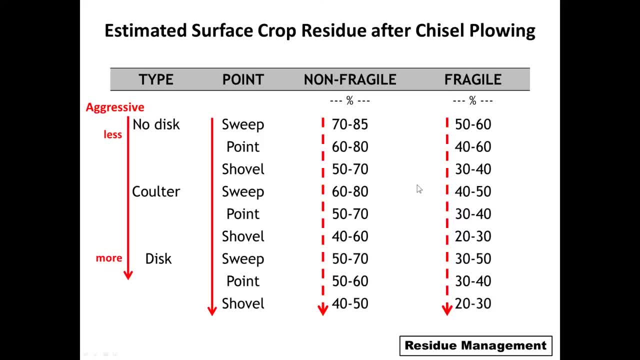 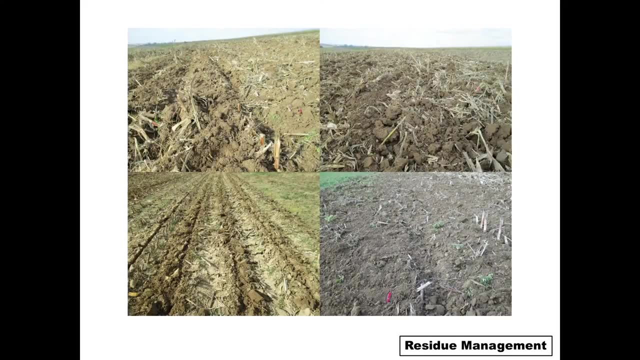 will leave more residue on the soil surface under both soil types And as you have a more aggressive setup, then you leave less residue on the soil surface. Here's another example: looking just visually at different tillage systems- I don't know you're looking at them. it would be hard to tell what they are. 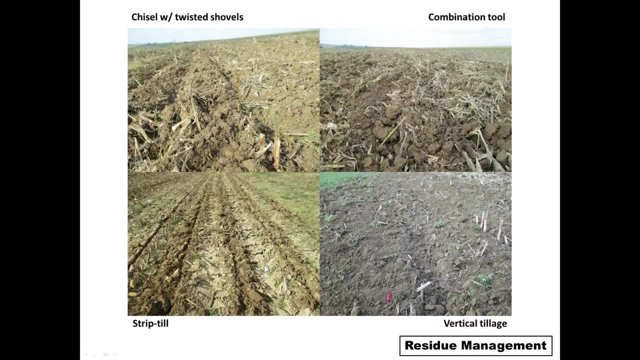 Maybe down in the bottom. here you can kind of guess. But here's what they are: Chisel Plow with twisted shovels, A combination tool. These are becoming very popular, especially in areas that may be more prone to compaction. 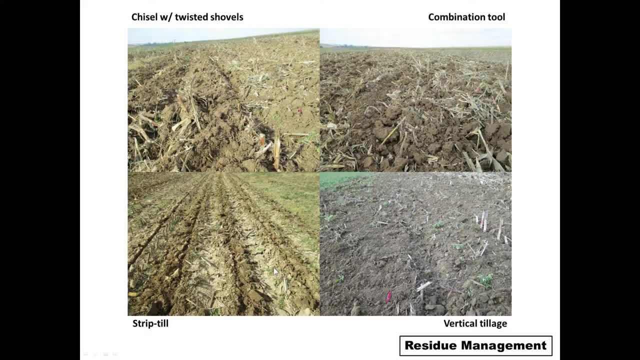 Strip-till. I think that's a great system where you have an area where you're preparing your seedbed, but then in between you have an area kind of similar to a no-till scenario, And here's a vertical tillage example where there was not a lot of residue on that field to begin with. 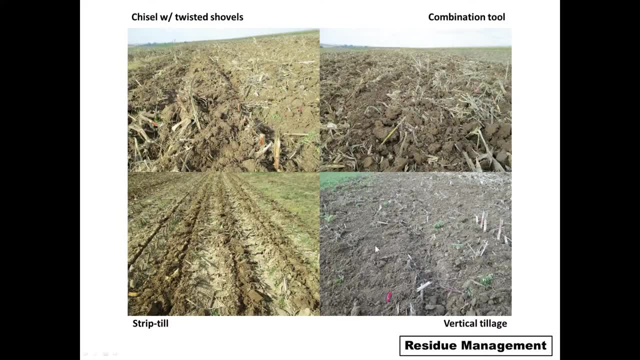 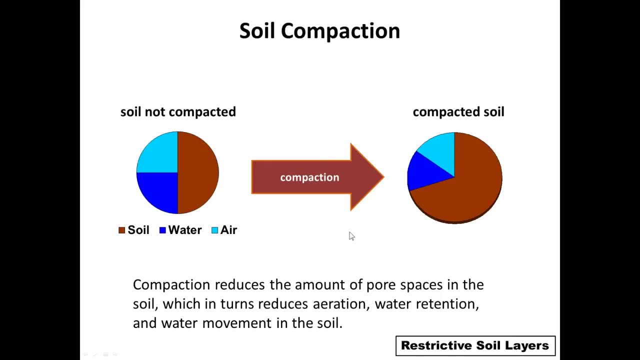 but you can see that it does a pretty good job of burying residue. I think it may be a little too good of a job because, just by looking at it, we have less than 30% left in this scenario. So let's switch gears a little bit and address some soil compaction issues. 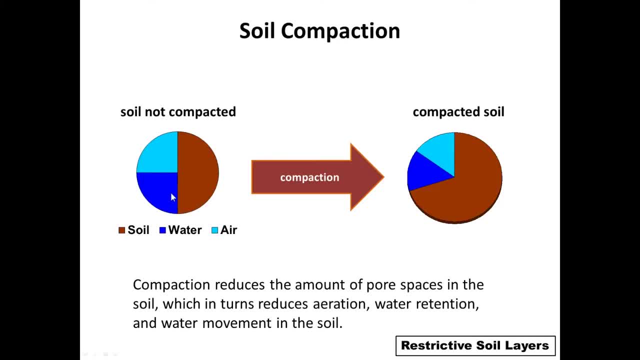 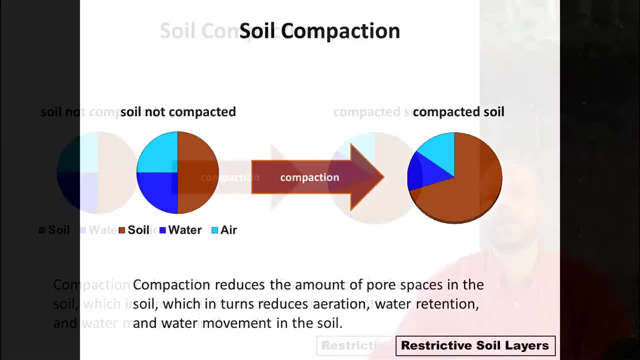 So if you look at the left on this graph, on this figure, here we have the soil not compacted. If you remember when we were talking about soil as a three-phase system, having the solid part and then the porosity that can be either filled with air or water. 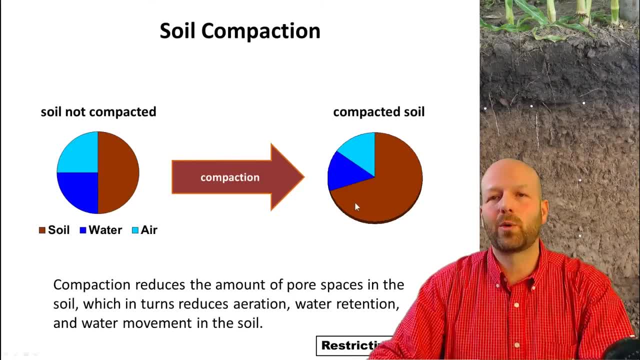 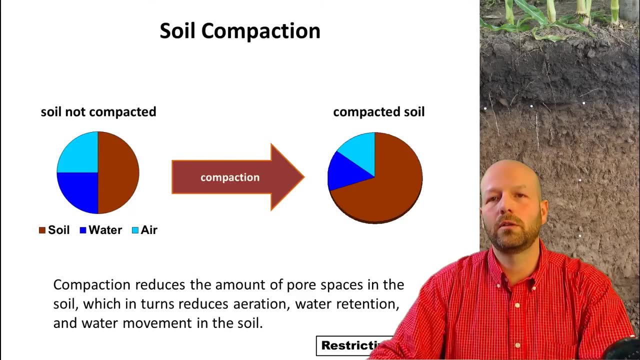 So what compaction essentially does is that it squeezes out the pore space out of the soil. So we have that soil basically squeezing out, or that soil occupying the solid part, occupying more of that volume of soil, and very little space left then for air or water to reside or to occupy. 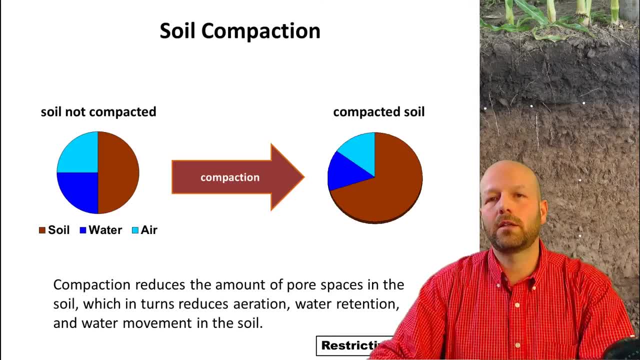 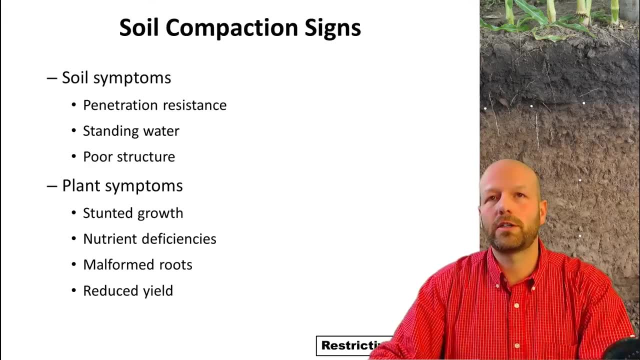 So obviously, as you can see, that will only not affect root growth, but it can also affect water relations in the soil. So what are the solutions? What are the symptoms or signs of soil compaction? So we're looking at the soil. 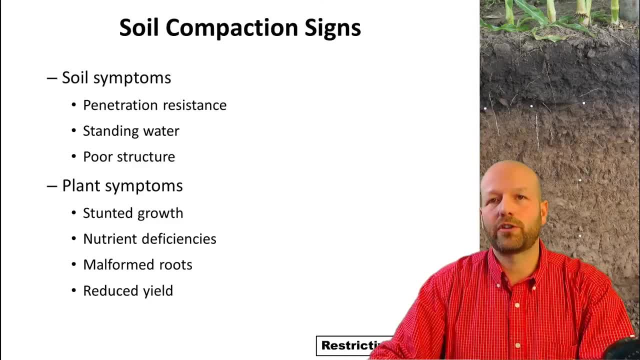 If we look at the soil, we can see that it would have greater penetration resistance. You can a lot of times see standing water on compacted soils. If you drive during a good rainfall event and look at fields, usually where water starts puddling is where you have your tire tracks. 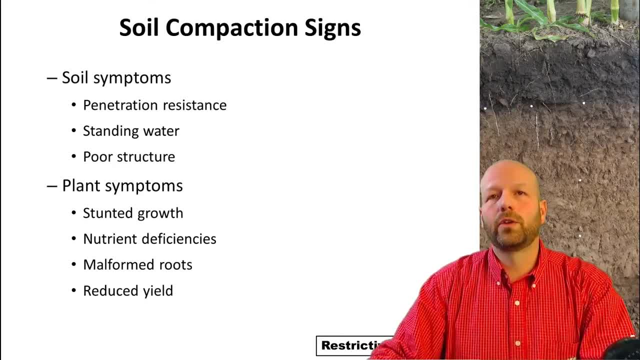 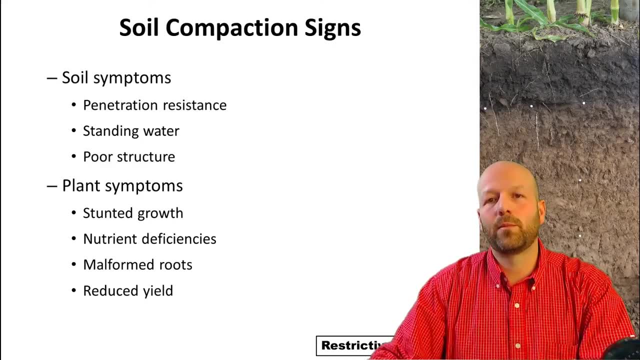 and those areas are the ones that tend to be more compacted, And also compacted soils are going to have poor structure. If you think about the different types of structure, the compacted soils will have more of that massive structure, So they won't have the blocky or the granular or the columnar type structure. 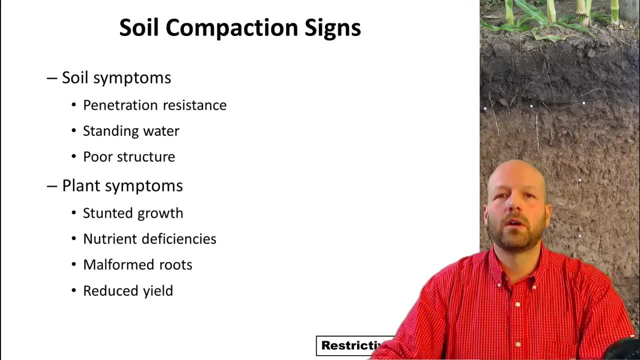 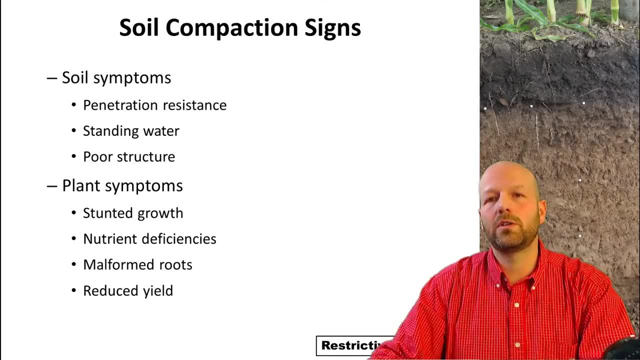 You can also look at plants to try to figure out if you have a compaction issue or not. So one of the effects is that you will see stunted growth. There might be nutrient deficiencies. One of the number one issues is reduction in potassium uptake. 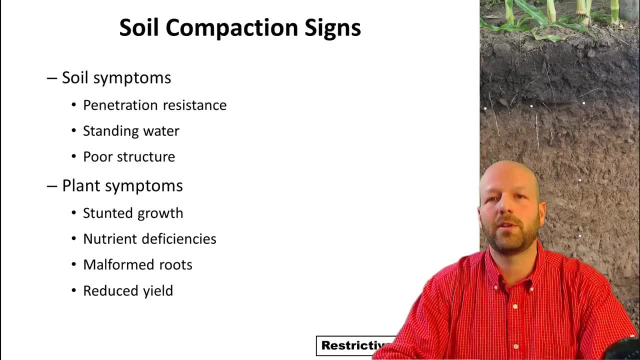 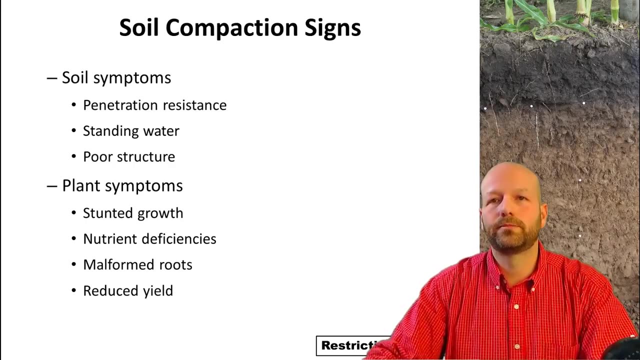 So the soil compaction can manifest itself as a potassium deficiency. A lot of times you will see roots that are not formed properly, They're not grown properly. So if you pull several plants and you look at them, you can see those signs on the roots and obviously a reduction in yields. 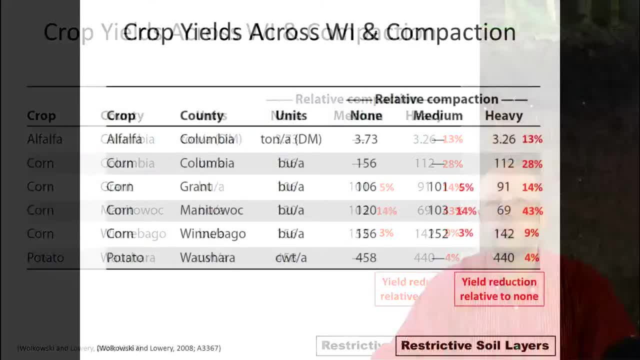 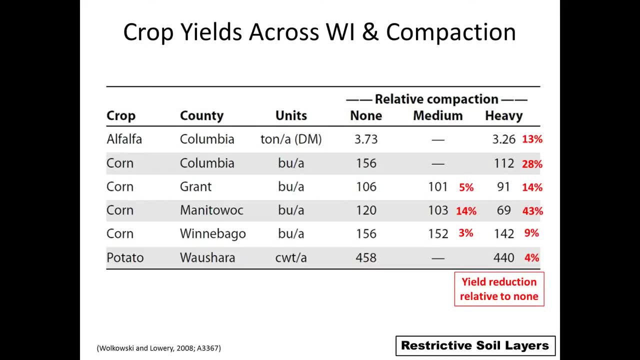 And here's an example of the impact on yield of compaction can have. So we can see different crops in different counties of the state and then different compaction levels going from north to south, From no compaction to medium to heavy. The numbers in red essentially tell you the reduction in yield relative to no compaction. 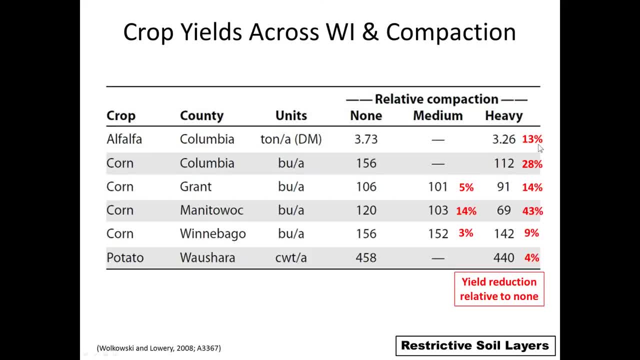 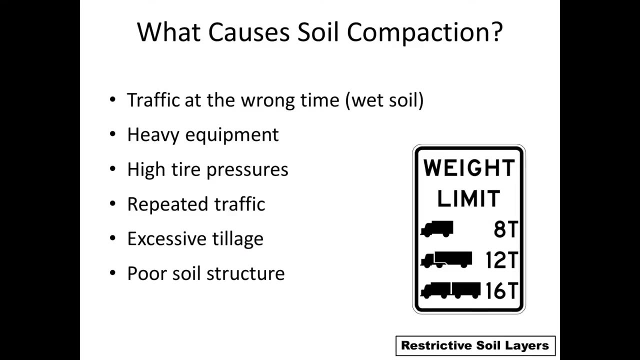 So here's an example of the top one: alfalfa: Reduction of 13% in yield. It can go as high as 43% in this case for corn. So a big issue for productivity. So in order to address compaction issues, we need to know what causes compaction. 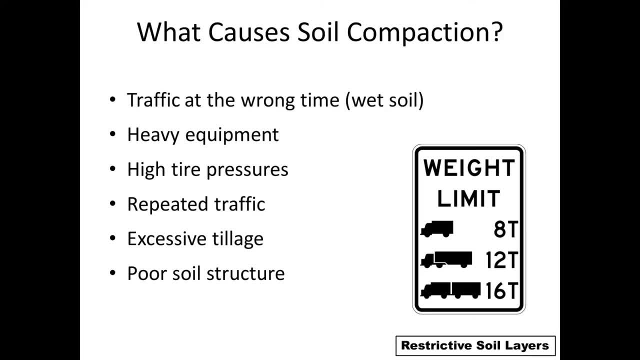 So what are the causes of compaction? So number one is the trafficking at the wrong time, And what I mean by that is getting out in the fields when they're too wet with our equipment. Essentially, what we're doing is crushing those aggregates in the soil. 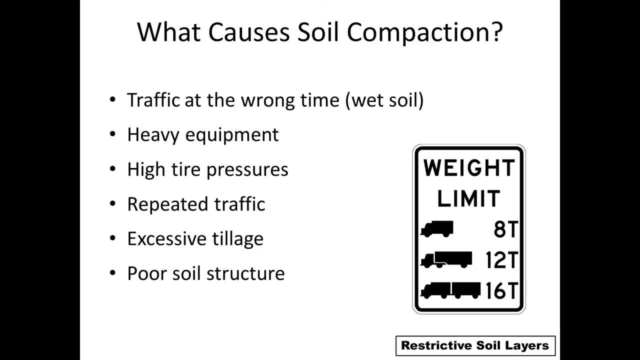 and squeezing again that pore space out. Another thing that's happening throughout the years is that equipment has been getting bigger and bigger and heavier and heavier, And so axle loads have increased tremendously in the last few decades And that actually has been contributing to. 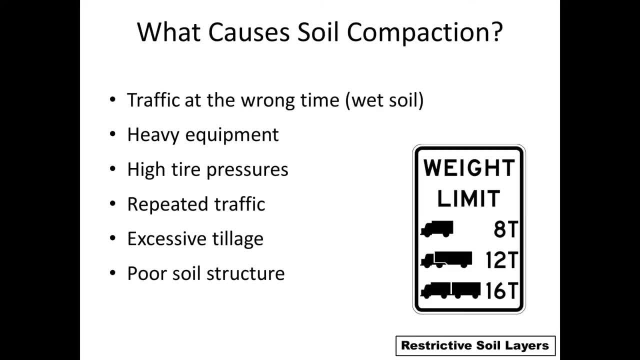 higher incidence of compaction. This growth in equipment relates to a lot of times with the shift that we be having in farms, where we need to farm larger areas in order to stay profitable, So it's just kind of a reality of things. Another issue that creates a lot of problem with compaction or increases compaction: 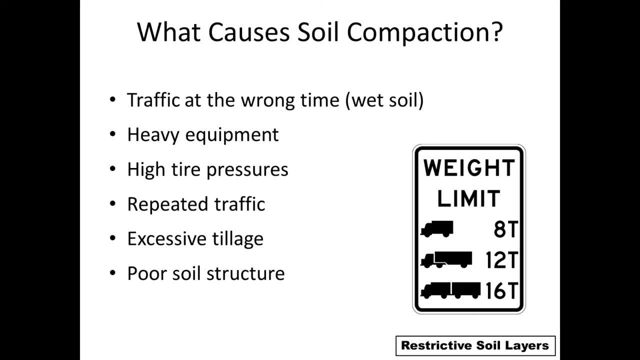 is running your tires with higher pressure than recommended by the manufacturer, So high tire pressures are a big, big problem. The other issue with that is that the higher your tire pressure, the less efficient your tractor becomes. You get more slippage. 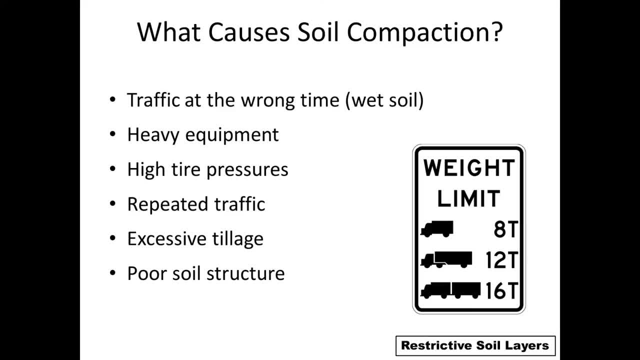 So that's a double whammy, So that actually it's important to look at tire pressure, Repeated traffic. it could be very harmful for compaction, create a lot of compaction, But have in mind that under the right conditions. 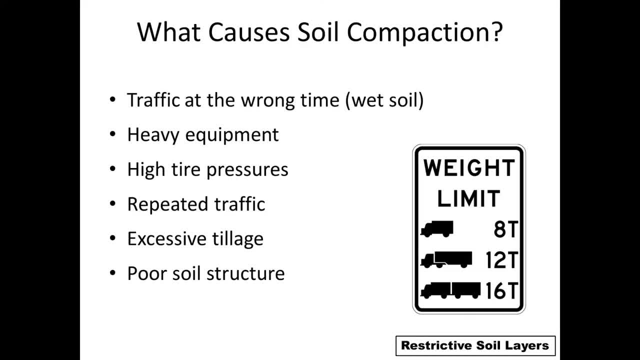 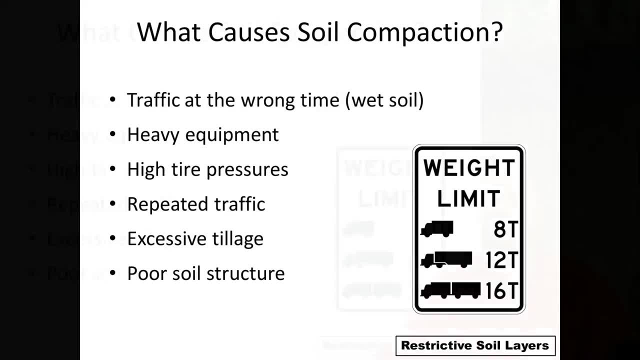 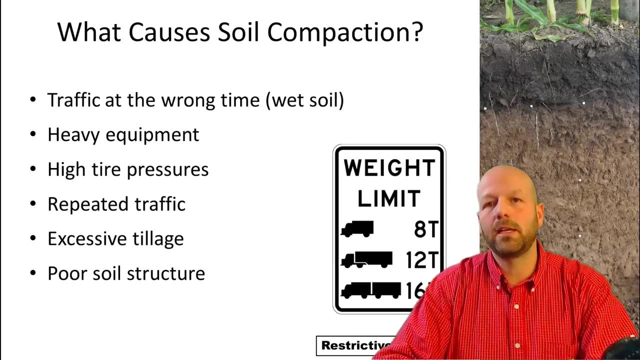 the first pass of a vehicle can cause up to 70% of that compaction. Excessive tillage can be a big problem. Every time we do any tillage operation we will be breaking some of the aggregation in the soil. So doing some tillage when needed not a big deal. 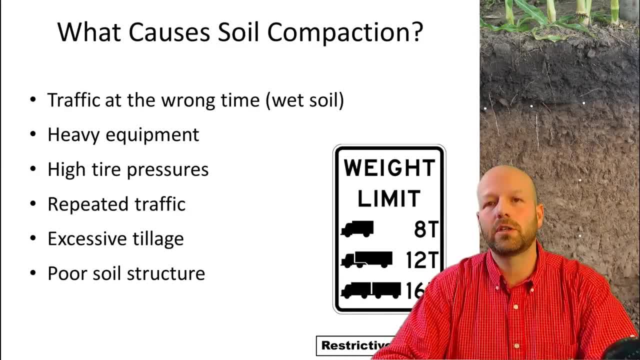 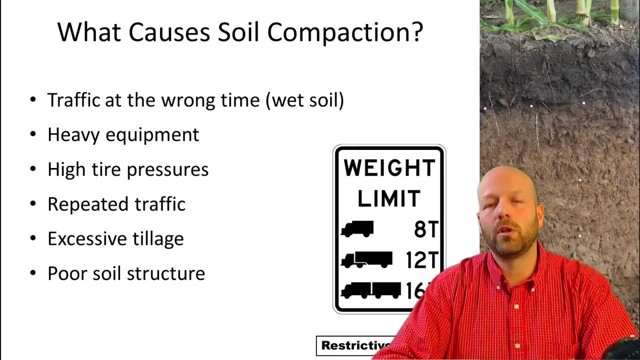 The soil can bounce from that. But if we do a lot of recreational tillage, that will cause problems with over destruction of aggregates and will really affect the aggregation of that soil. Once that soil has lost its aggregation it will be a lot more susceptible to 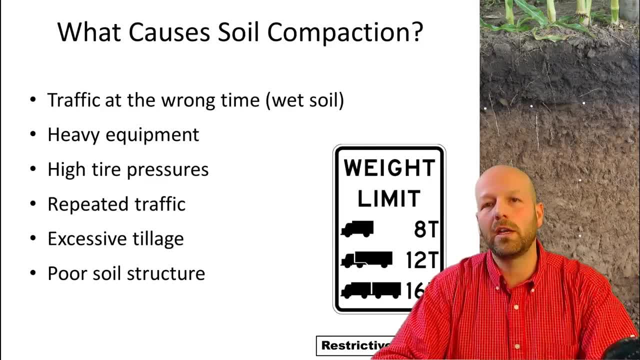 uh, compaction. Think about a recently tilled field. If you go walking in that field right after tillage, what happens? You actually sink in that field. So that field essentially has lost its ability to hold the load. And so, again, that goes to the next point in here. 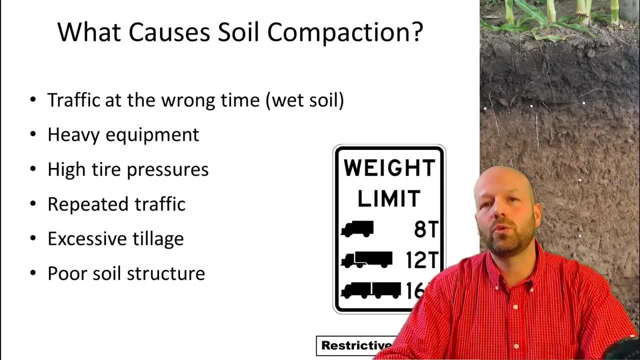 which is the poor soil structure Again. so any management that you can do to improve soil aggregation, soil structure, such as use of manures, cover crops- all those things that we have talked about in the past- will help with compaction management. 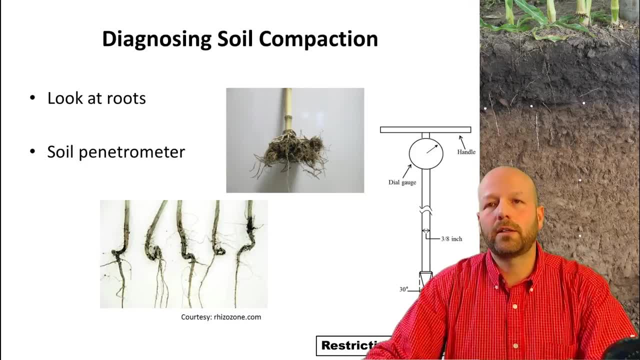 So talk briefly about the diagnostic soil compaction. So the two most effective ways, I think, in my view, to do that it's looking at roots. Here's an example of a corn root, what typically we call the pancake root system. 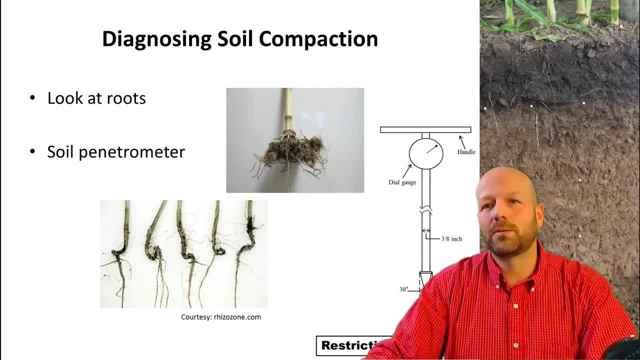 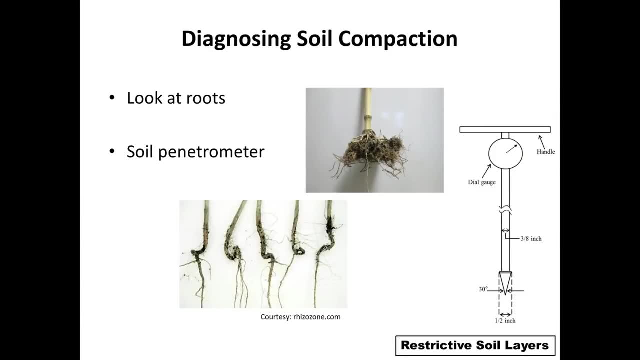 That's a technical term right. So this is more indicative of shallow compaction, where the roots are not able to penetrate the soil deep. in the profile We're looking at a tap-rooted type crop, such as soybean. We see what we call jade rooting. 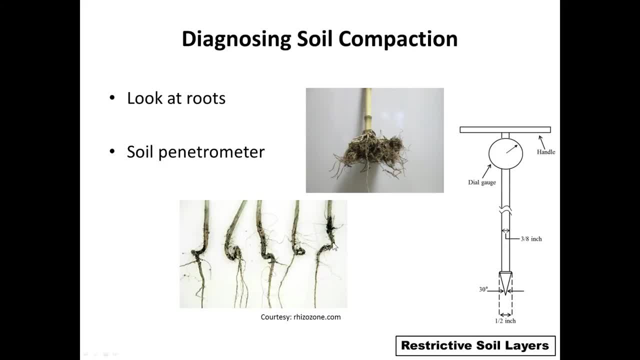 So the tap root is actually trying to penetrate that compacted layer but then cannot penetrate and so it goes laterally to try to find an area of least resistance, And so it tries to keep doing that and we can get this really odd-looking root system. 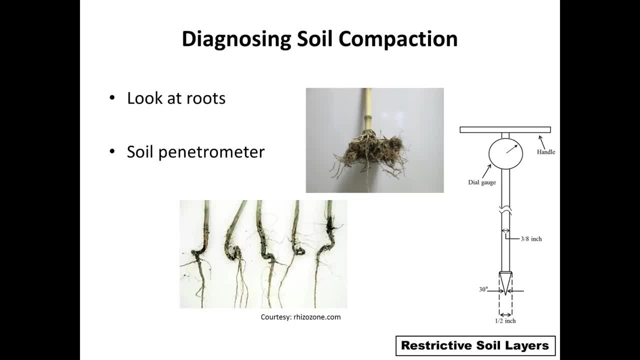 Another good tool for assessing soil compaction is use of the penetrometer. Here's a schematic of a soil penetrometer. Essentially, it's just a stainless steel rod with a pointy end And we push that into the ground to give us an idea. 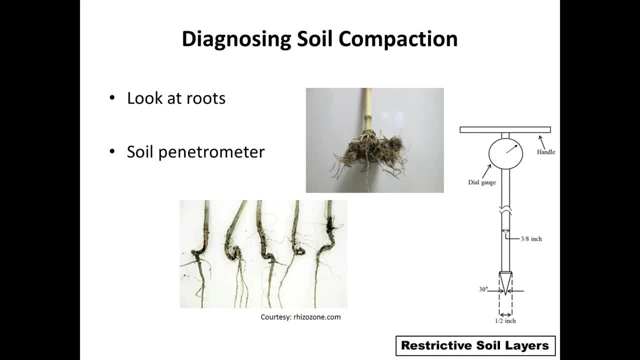 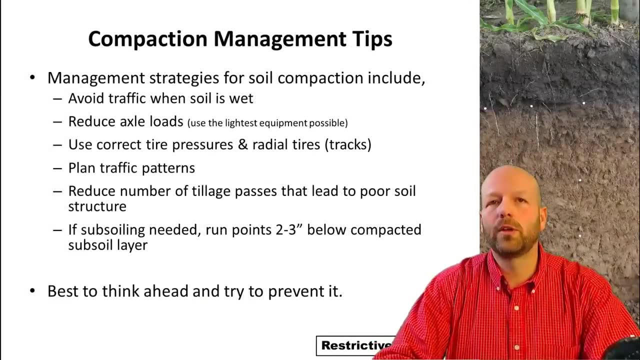 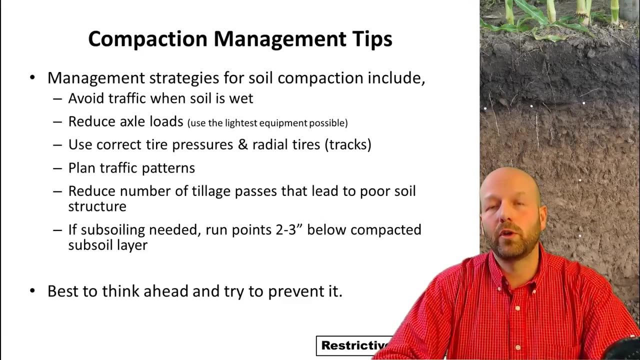 of the relative bulk density of that soil and assess the compaction status of that soil. So a couple of tips on soil compaction. So things that we can do to management compaction would be to avoid traffic when soils are wet. try to reduce the axle load. 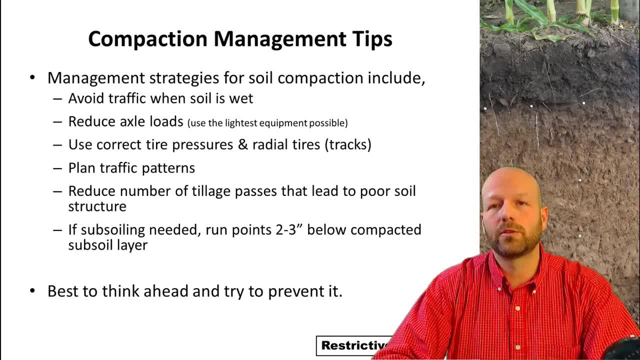 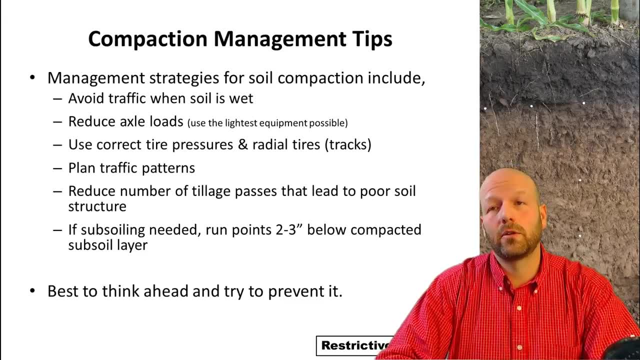 So a way to think about it is to try to use the lightest equipment when possible, so not if you're having to do a certain task, can you do that with a smaller tractor? Use of radial tires or tracks in a lot of scenarios can be useful. 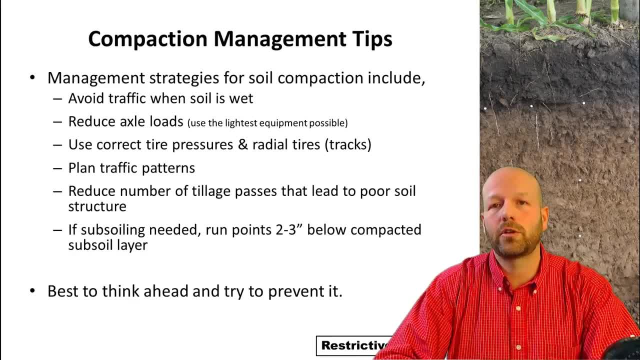 but keeping those tires at the right pressure. it's crucial. The other thing, too, is to maybe plan ahead the traffic patterns in the field. A lot of people are going to control traffic. maybe don't need to go to that level of management. 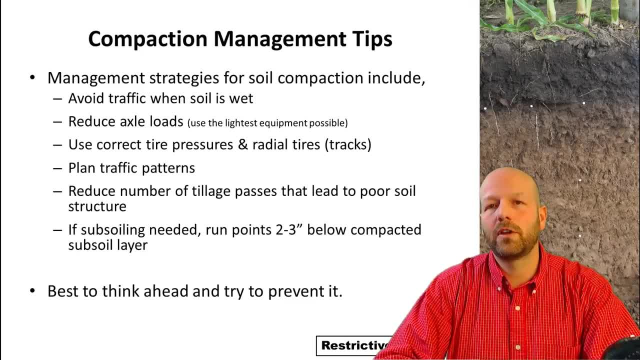 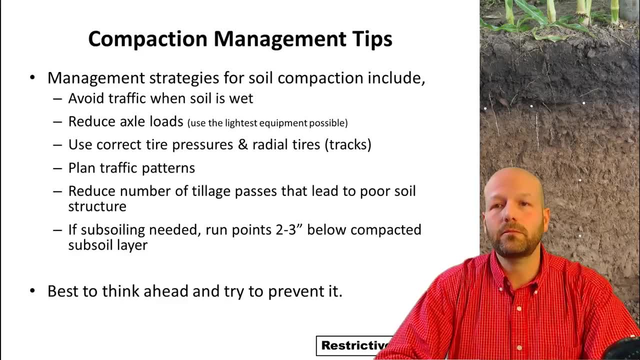 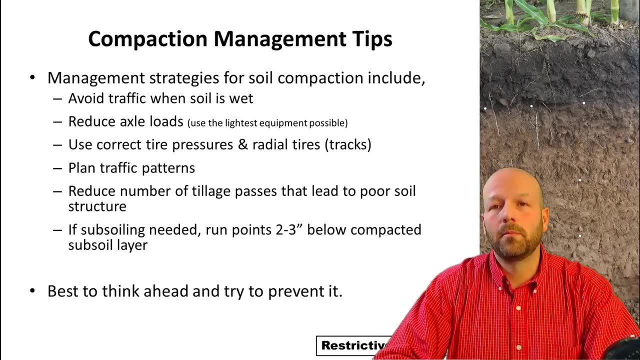 but planning certain traffic operations through the field could be beneficial. Also, reduce the number of passes. This could be beneficial in reduced compaction And a lot of times we might have subsoil compaction and that is needed to improve the rooting conditions. 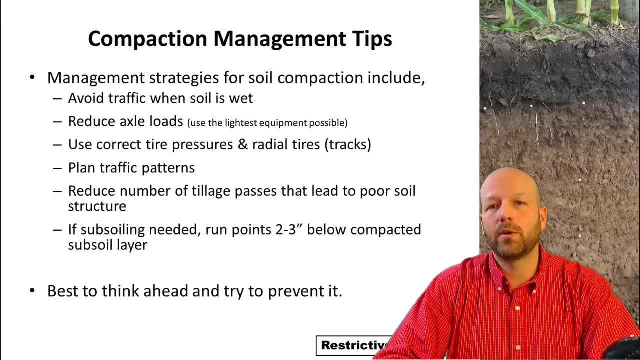 So, if that is needed, just have in mind that the most effective way of running a subsoiler is to run the point of that subsoiler two to three inches below the bottom layer of the subsoil compacted layer, And a way that I like to think about a subsoil compaction. 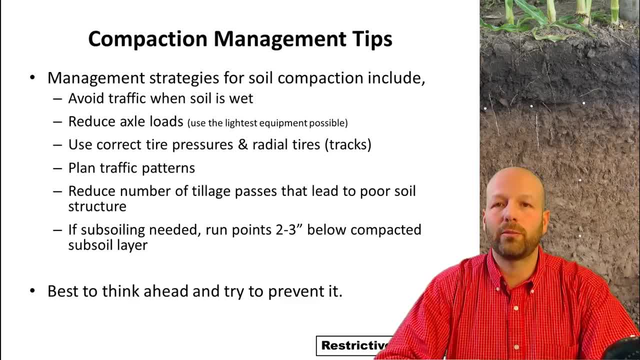 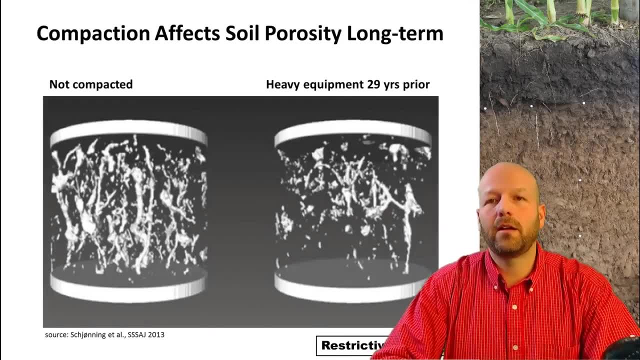 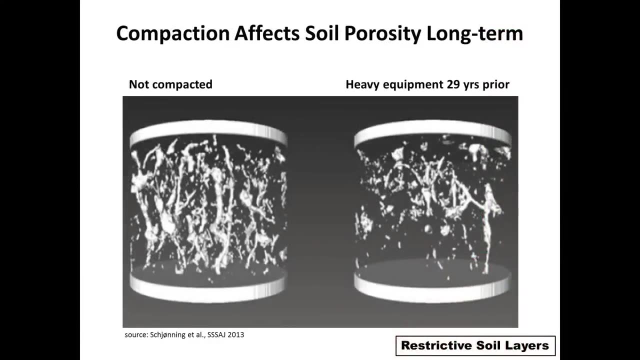 is that it's better to think ahead and try to prevent it than try to remediate or eliminate it in the future. And here's an example of that. This is a computer tomography or CD scan of subsoil samples down to one foot. 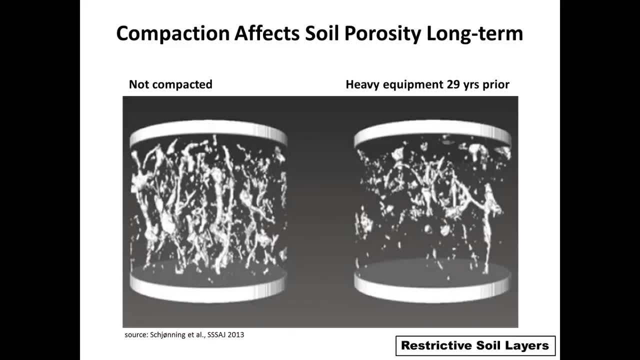 And this was done in a research scenario where these researchers had done subsoil compaction 29 years prior to taking the course. So we see on the left, a non-compacted area, And so what we're seeing there? all those little lines in there. 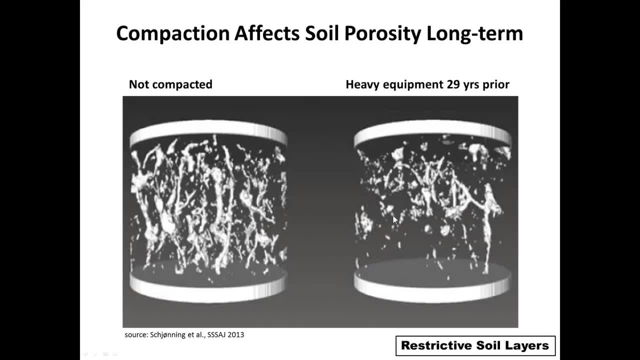 that's actually macro porosity, or porosity in the soil. And then you can see on the right that's actually the compaction done 29 years before that And you can see after 29 years you can still see the effects of that compaction in there where the aggregation of that soil has been affected. 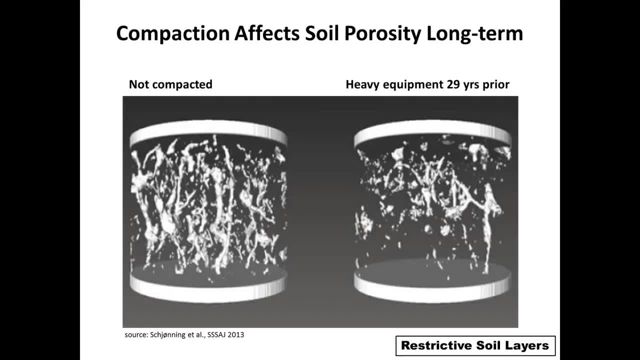 So this, to me, highlights two things: is that compaction will not go away on its own. These two soils were actually treated the same way, managed the same way. But it also highlights that if you do have subsoil compaction, subsoiling can be quite effective at managing that issue. 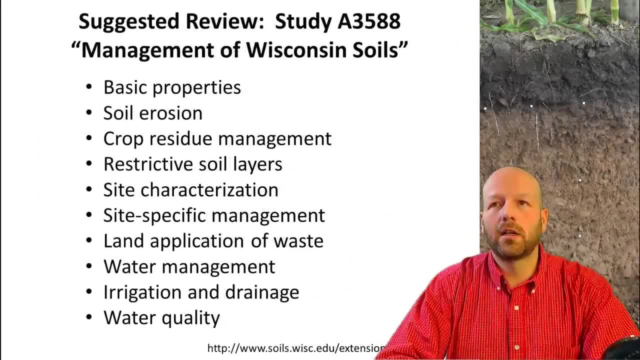 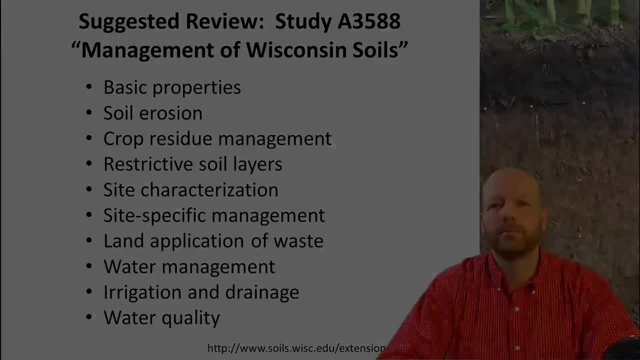 If you need a little bit more information in detail, I direct you to the 83588 publication- Management of Wisconsin Soils- www.83588.com.